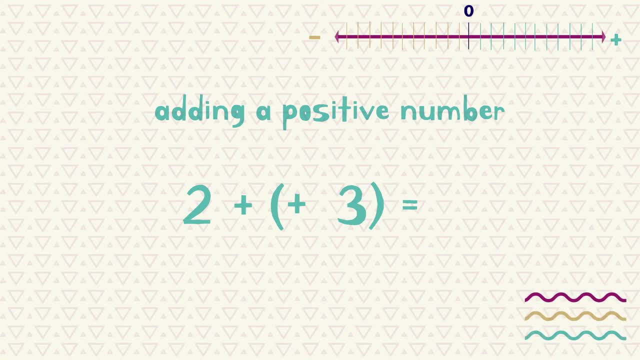 3 to the number 2.. Sometimes the number may or may not be shown with brackets, As we are adding a positive number, are essentially just adding. So the rule is that when we have two plus signs together, we can just change this to a single addition sign. So why is this? 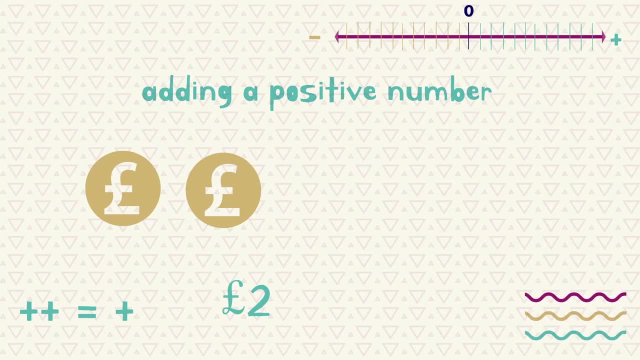 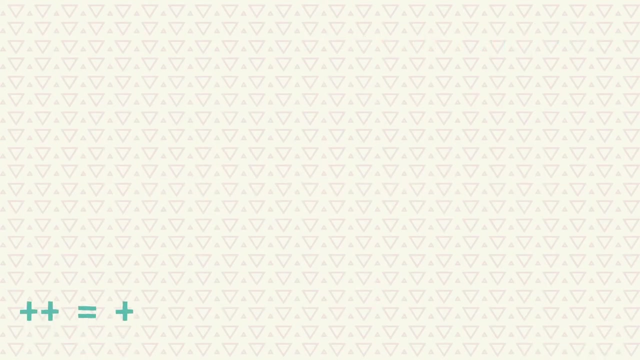 Imagine you have two pounds in your bank account and you want to add a positive amount of three pounds to your account. You are really just adding three pounds. Let's look at this same example. on the number line We start with the number two and we add a positive amount of three and end up at five. 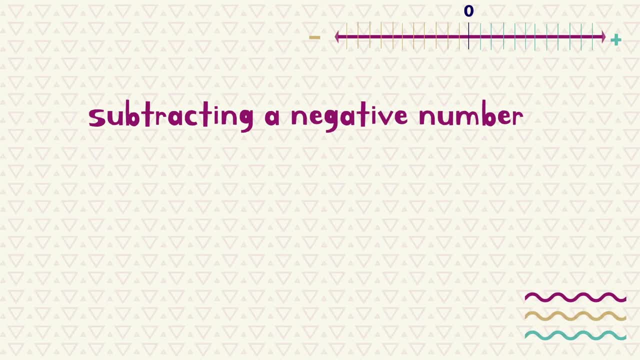 Now let's look at subtracting a negative number. Here we are subtracting a negative three from the number one. The rule is, if you are subtracting a negative number, you are actually just adding, So you can change the two signs to an addition sign. This may sound confusing, so let's look again at a real 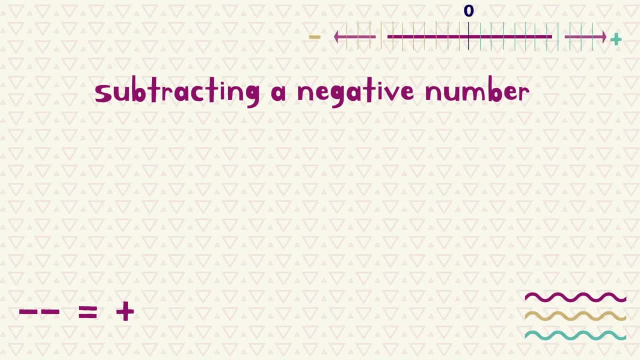 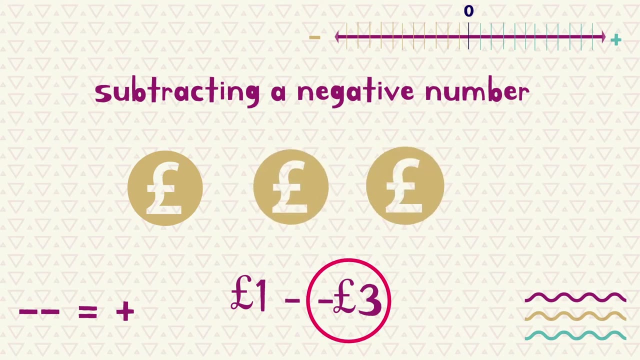 world example. Imagine you have four pounds in your bank account. Now the bank accidentally takes away three pounds. so now you are left with one pound To undo their mistake, or in other words, change the number three to a negative three. you have to add three pounds back to your account. 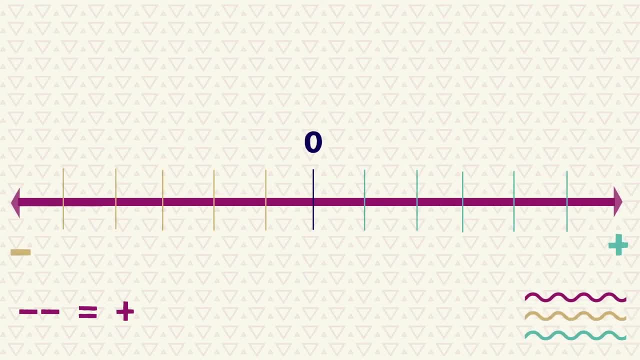 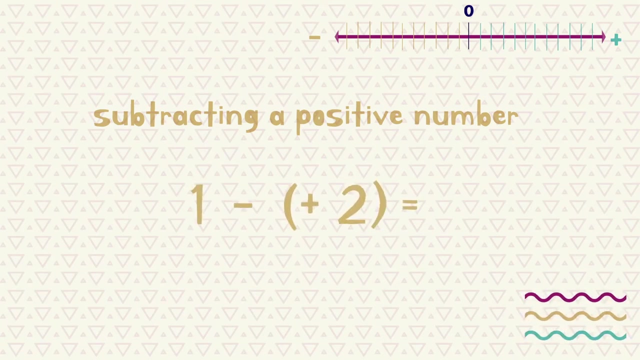 Let's have a look at this on the number line. So we start at one and because we are actually just adding the three, we end up at four. Now let's look at subtracting a positive number. In this example, we are subtracting a positive two from the number one. 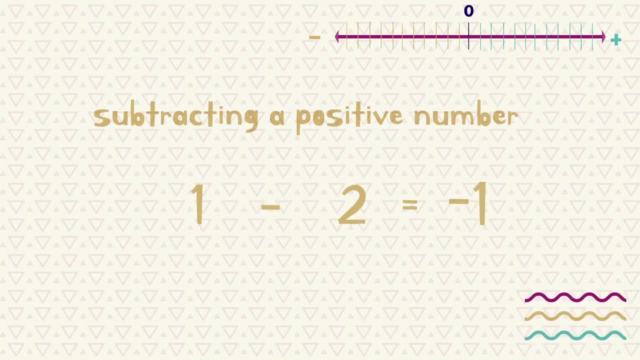 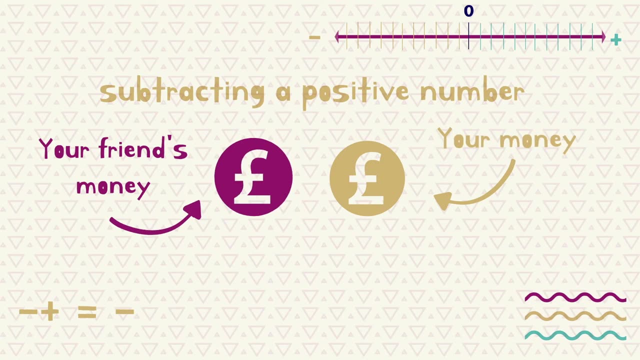 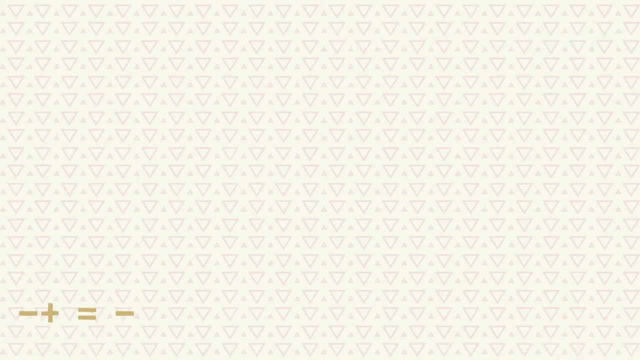 Essentially, we are just subtracting, Thinking of this in terms of money. Let's say you have one pound, but you want to buy something that is two pounds, So you borrow one pound of your friend's money. You now owe your friend one pound, so you are left with minus one pound.